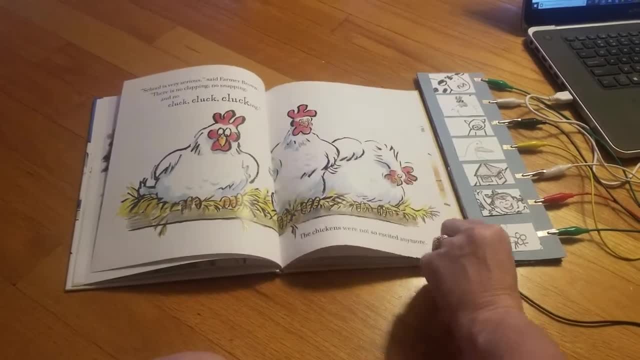 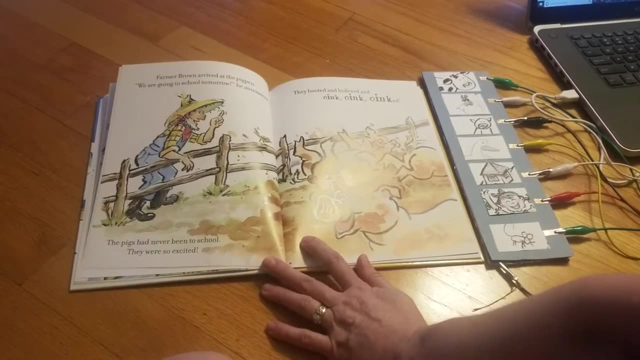 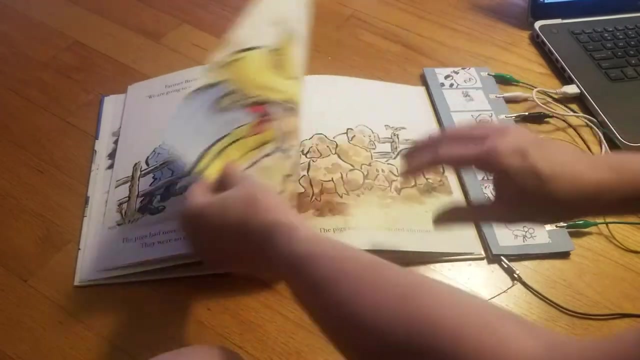 mooing, The chickens were not so excited anymore. Farmer Brown arrived at the pig pen. We are going to school tomorrow. he announced The pigs had never been to school. They were so excited. They hooted and hollered and mooed. School is very calm, said Farmer Brown. There is no hooting. 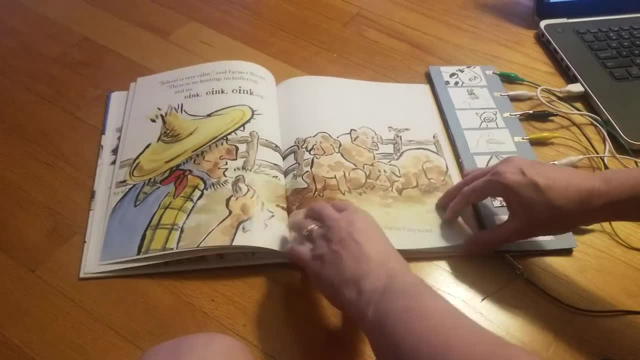 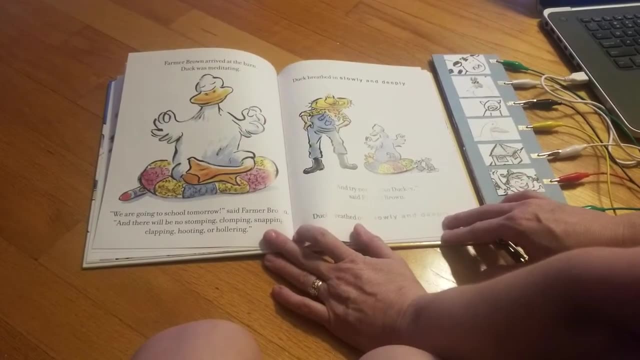 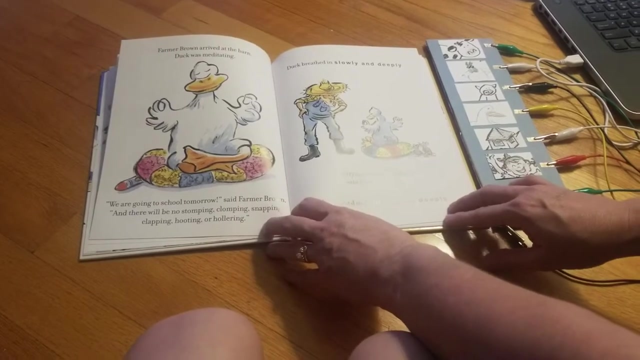 no hollering and no mooing. The pigs were not so excited anymore. Farmer Brown arrived at the barn. Duck was meditating. We are going to school tomorrow, said Farmer Brown, and there will be no stomping, clomping, snapping, clapping, hooting or hollering. Duck breathed in slowly and deeply. 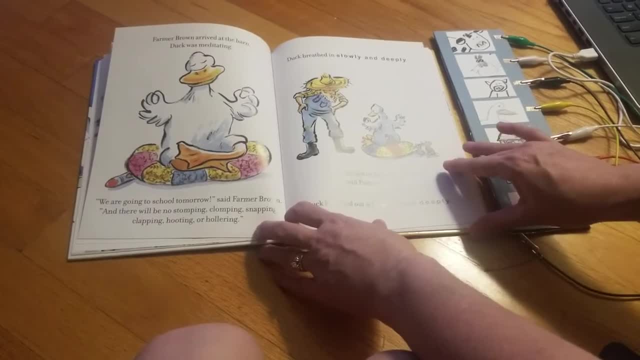 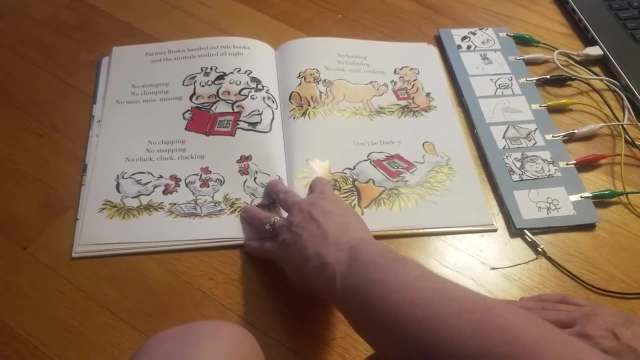 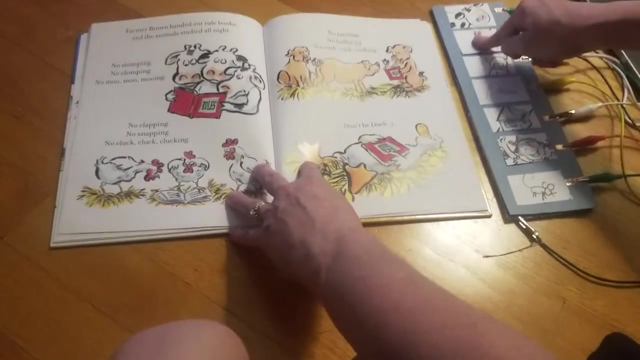 And try not to be so ducky, said Farmer Brown. Duck breathed out slowly and deeply. Farmer Brown handed out rule books and the animals studied all night. No stomping, no clomping and no mooing. No stomping, no clapping, no snapping, no mooing, No hooting, no hollering, no mooing And don't be. 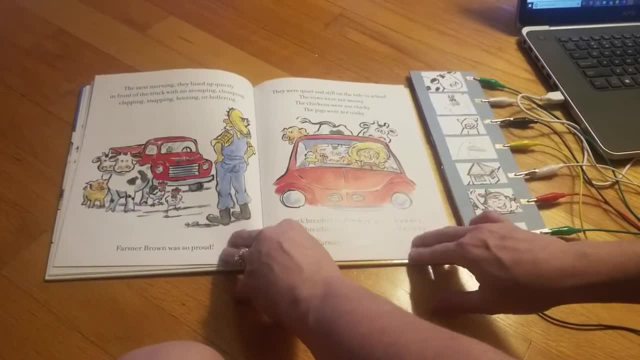 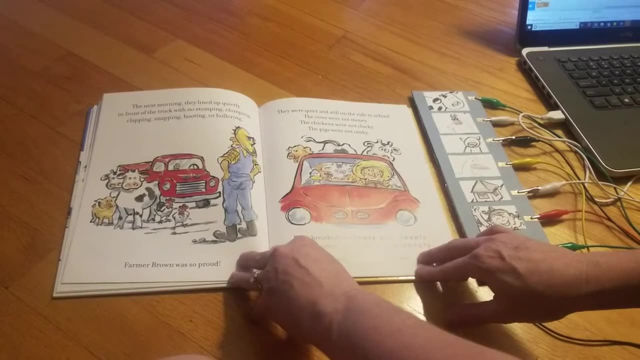 ducky. The next morning they lined up quietly in front of the truck with no stomping, clomping, clapping, snapping, hooting or hollering. Farmer Brown was so proud They were quiet and still on the ride to school. The cows were not, The chickens were not. 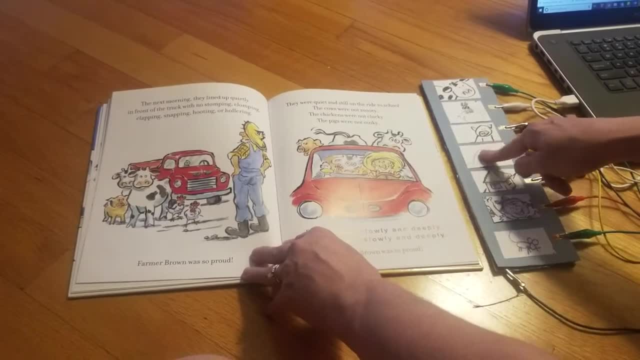 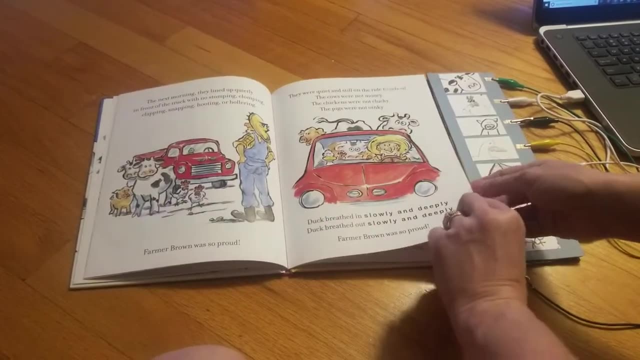 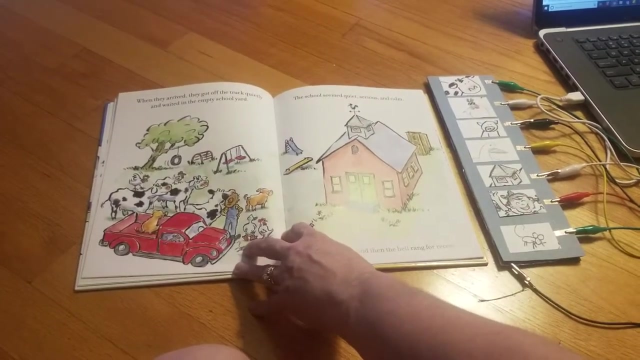 The pigs were not. Duck breathed in slowly and deeply. Duck breathed out slowly and deeply. Farmer Brown was so proud. When they arrived they got off the truck quietly and waited in the empty schoolyard. The school seemed quiet, serious and calm. 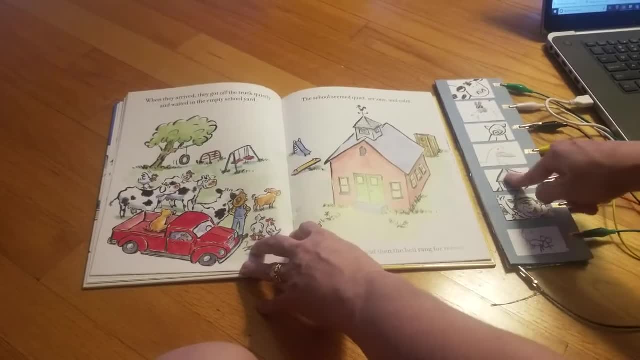 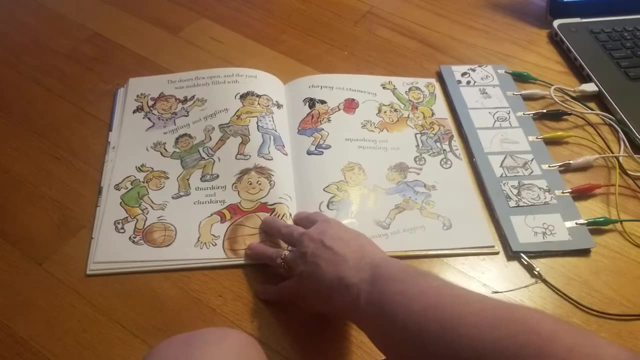 And then they heard the bell. and then the bell rang for recess, The doors flew open and the yard was suddenly filled With wiggling and giggling, thumping and clunky chirping and chattering, squeaking and squealing. 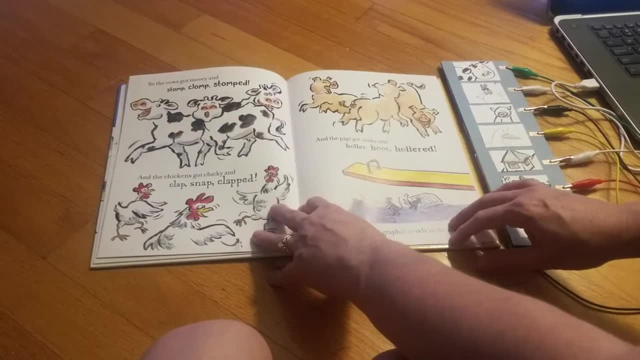 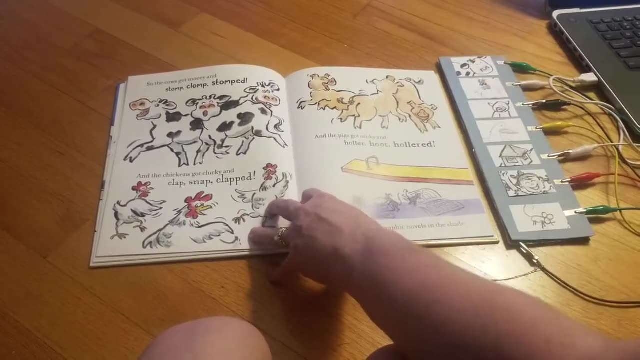 and zooming and zigging. So the cows got mooing and stomped, clomped and stomped, And the chickens got clucky and clapped, snapped and clapped, And the pigs got oinky and holler.